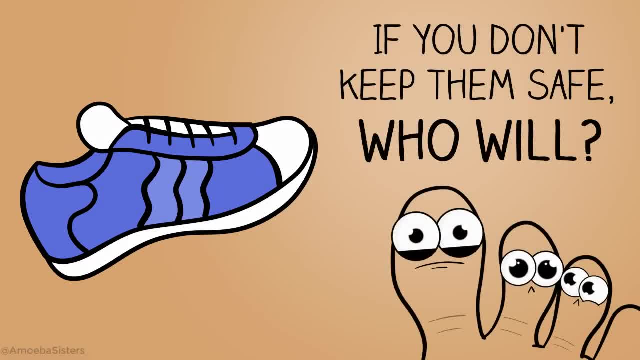 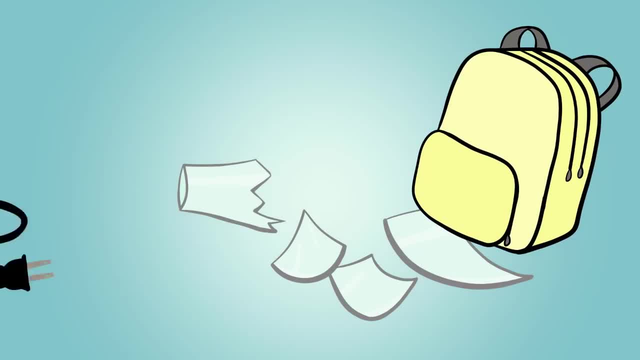 You should wear closed-toed shoes because you don't want to be pouring something toxic on your feet Or walking on broken glass. Speaking of broken glass bags and stuff in the aisles and lab rooms do not help. You want a clear path and not have your belongings out where someone could. 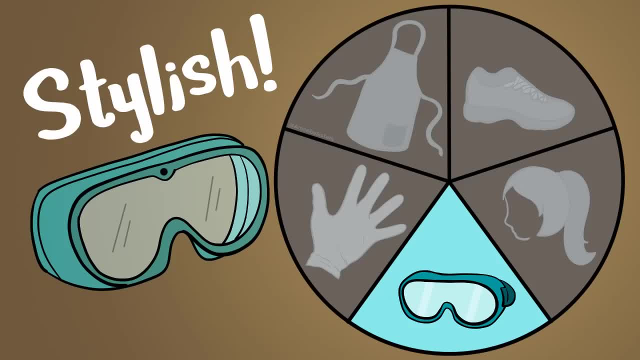 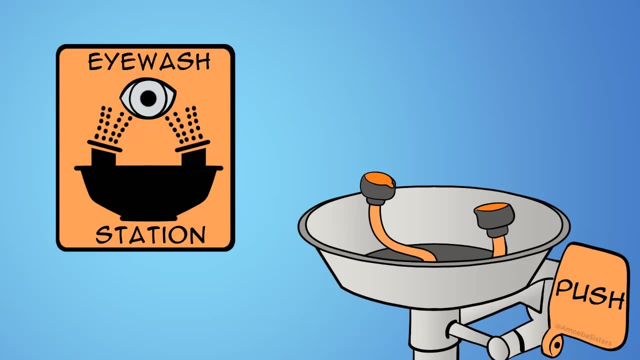 trip over them. And no horseplay. To protect your eyes, wear goggles. And when we say wear goggles, we all know that on your forehead doesn't count. If you do feel as though something has gotten in your eyes, you will want to use the eyewash station, which will require you to hold 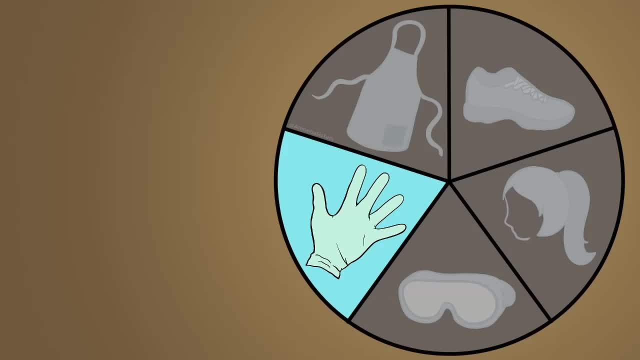 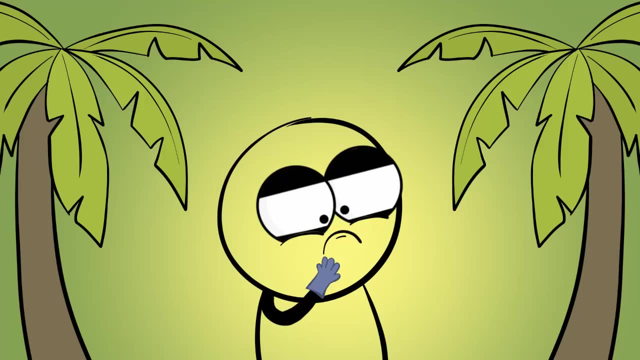 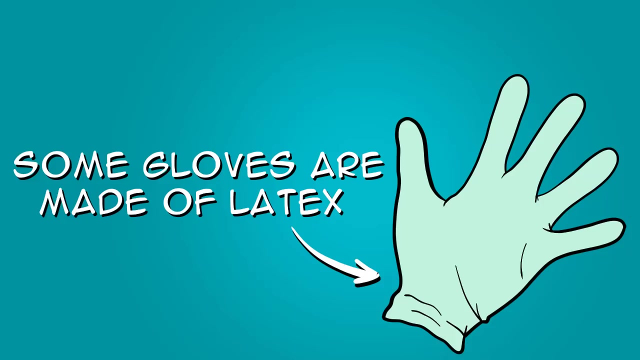 your eyes open under the running water. If your lab involves working with specimens or chemicals, you will likely be advised to wear gloves. Gloves are important. Yes, sometimes they make your hands feel clammy, but you know what's worse- Chemicals that can irritate or burn your skin. If you have an allergy to latex, you should make 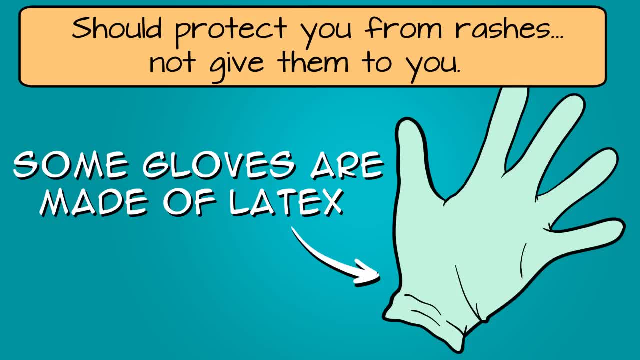 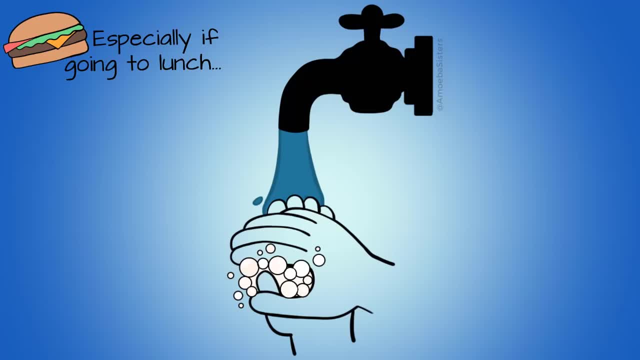 sure that the gloves you are using are latex-free. Ask your instructor. In fact, if you have any allergies, you should let your instructor know When you finish a lab. even if you wore gloves, it's a good idea to wash your hands after time in the lab. Some labs may require you to wear an. 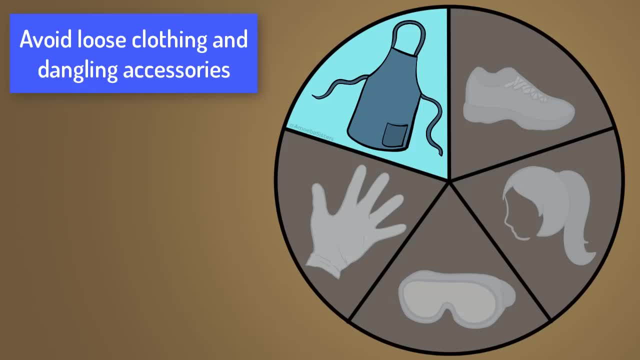 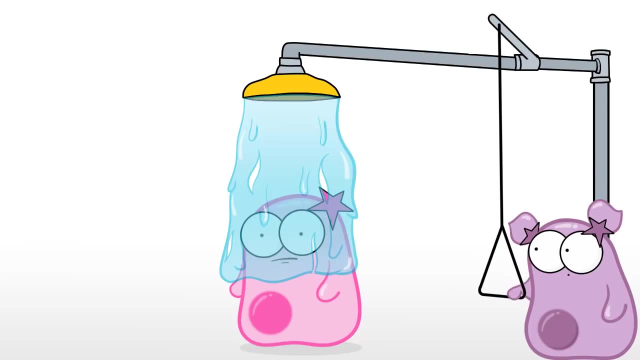 apron to protect your clothes. Depending on what type of course you are in and the type of labs you are doing, you also might have a safety shower, which will double your ability to clean up your face. If you have an allergy to latex, you should be careful not to wear gloves. 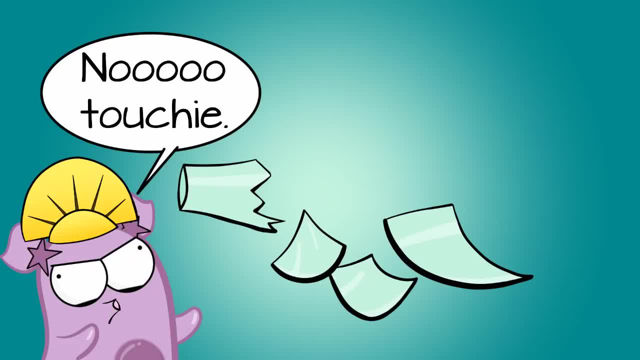 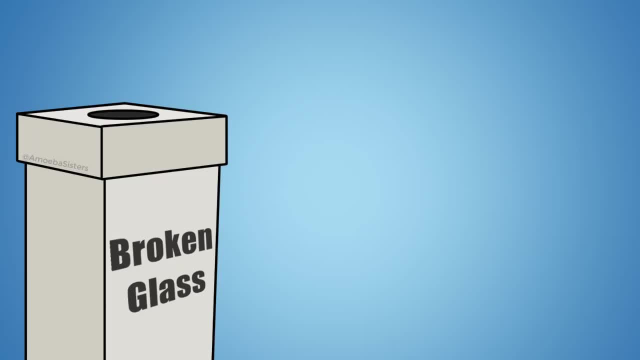 If you accidentally break glassware, don't pick it up. It could cut you. A broom and a dustpan should be used to clean it up And there should be a place designated for broken glass, Not the regular trash, where it would just break through the trash liner. If you see glassware that is chipped already. 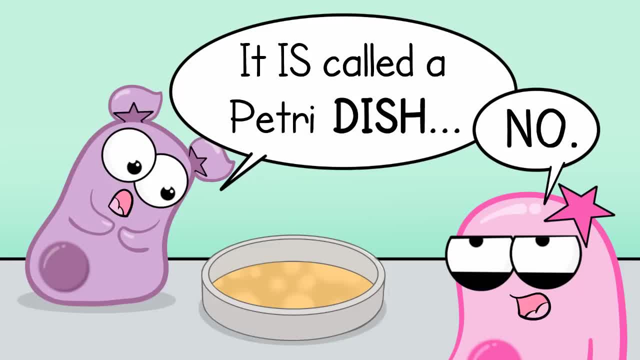 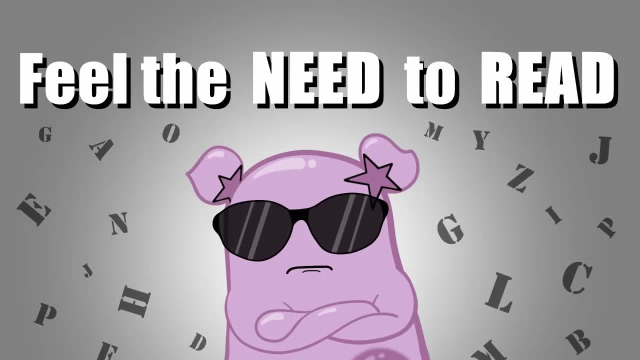 don't use it and tell your instructor. Never drink or eat anything in the lab. That includes chemicals. Don't taste or smell chemicals. Don't drink or eat anything in the lab. Don't eat or smoke chemicals. Read labels. Don't ever pour chemicals that you may be using back into the. 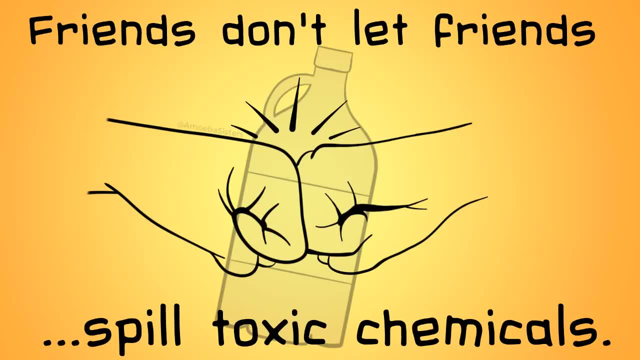 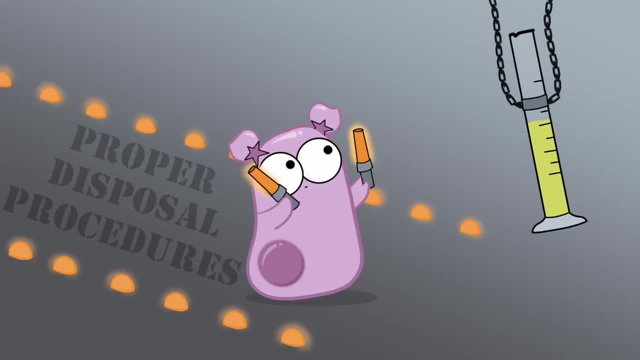 bottle that they came from. As soon as you finish pouring chemicals out of a container, the container should be immediately closed. When you're done with a chemical, you want to make sure you properly dispose of it. Many chemicals can't just be put down the drain. In fact, some 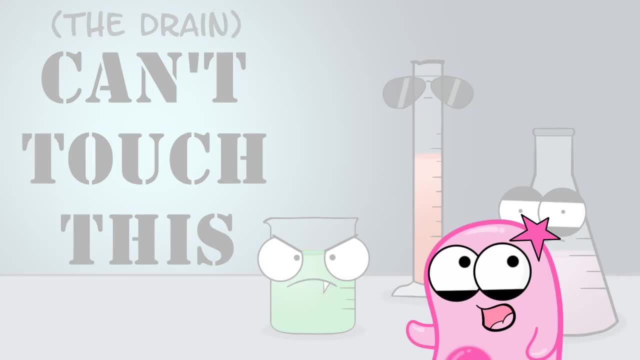 solid items that you use in your labs also cannot be thrown away in the regular trash and have to be disposed of as hazardous. If you have a lot of chemicals in your lab, you should be careful not to use chemicals that are hazardous waste. Always check with your instructor. 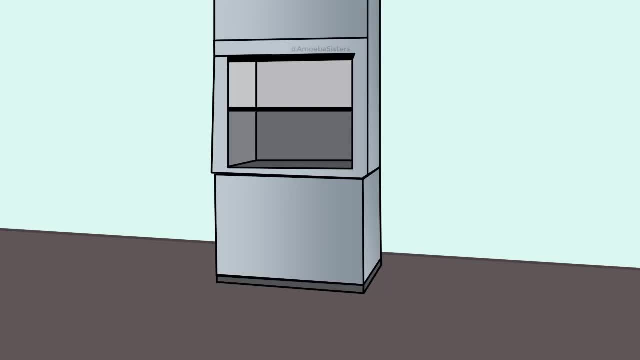 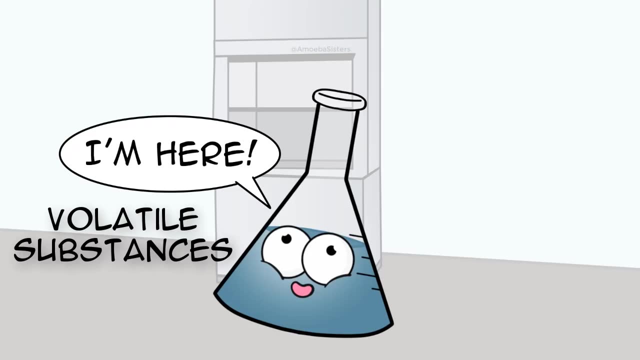 In some labs, you may have a special ventilation system, also known as a fume hood. This is used when dealing with volatile substances, which is a fancy way of describing a substance that can easily vaporize. Some of your labs may require the fume hood because some of these 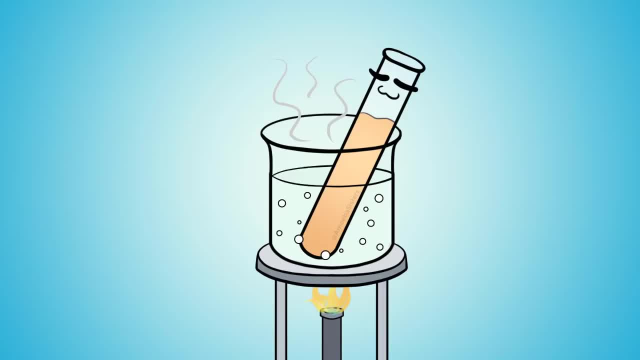 volatile substances may be harmful if you inhale them. When you're heating things up, like this test tube in a hot water bath, don't have the test tube pointed towards you. Use it when you're using tongs or heat protective gloves to handle the test tube that you may be heating. 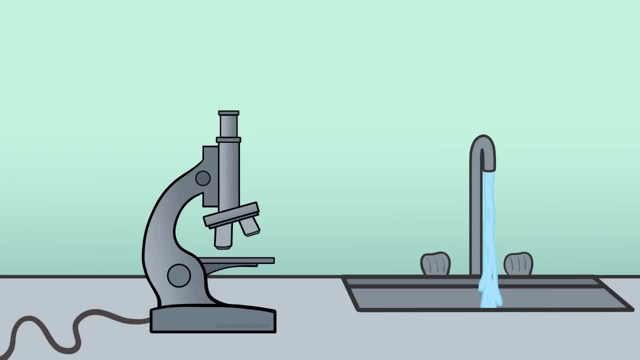 Also, electricity and water are not a good mix, So when you're doing your super awesome microscope lab, you want to keep the water away from the electrical cord. And speaking of microscopes, we could have an entire video on just working with the microscope, But for now we'll make 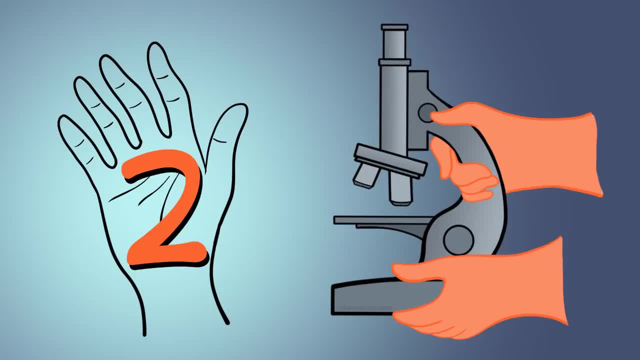 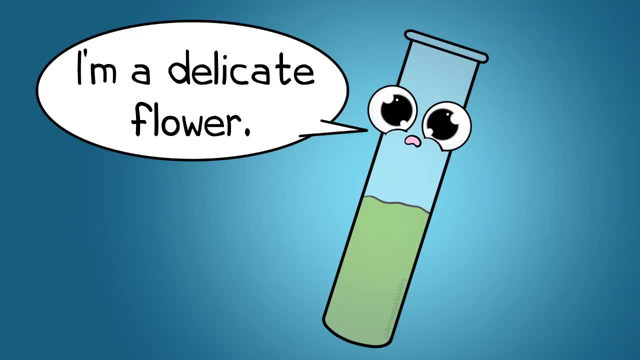 sure to mention carrying it with two hands: One hand underneath the base and the other holding the microscope arm. If you're using any special science equipment, you might want to make sure to use a streaml challenged this time. Here's an example of how to do this. 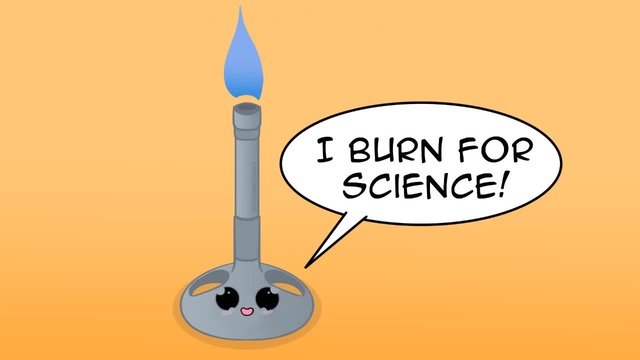 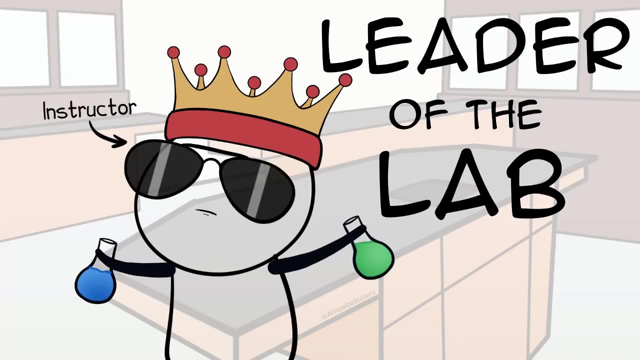 If you are in a lab that has an open flame, obviously be aware of the flame Review with your instructor how to operate the valve that controls the gas fueling. the flame Review with your instructor how to properly heat the various glassware that will be suspended. 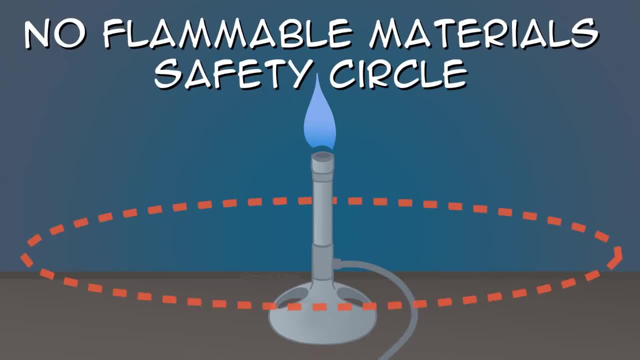 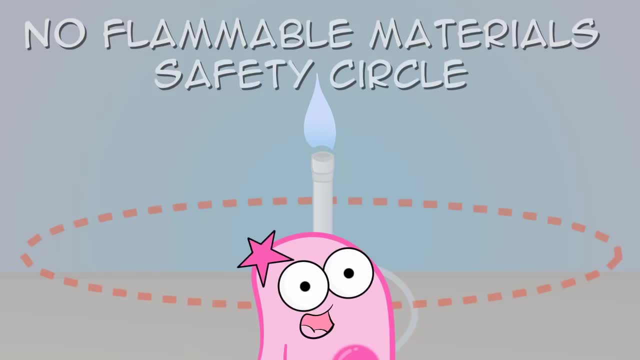 over the flame. Every time you are in the lab with an open flame. you must keep all materials that may be flammable away from the area near the flame. Depending on the types of labs you're doing, your lab room may also have a fire extinguisher. that is. not visible, The numerous glassware and the flammable flammable material could be damaged. Also, if your lab is used to be friendly to the fire, you might not want to teach the staff. A fire extinguisher can serve as a fire extinguisher. If you're using a flammable fire extinguisher. 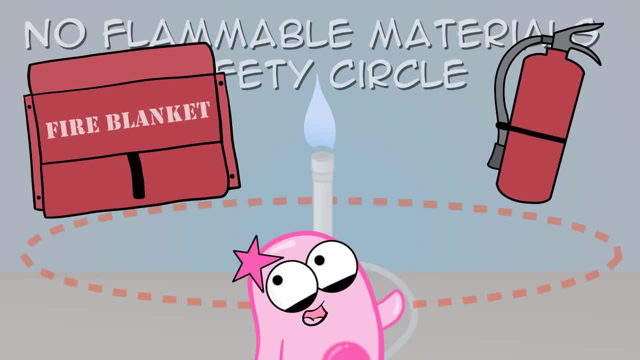 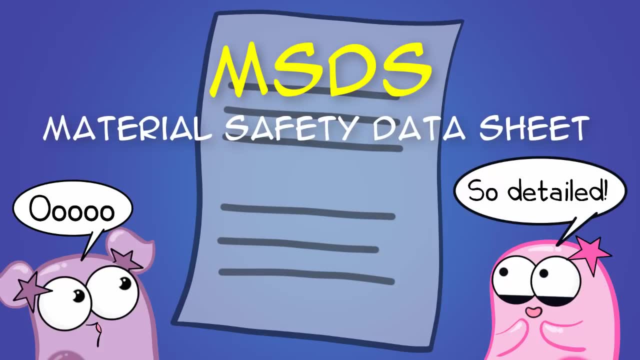 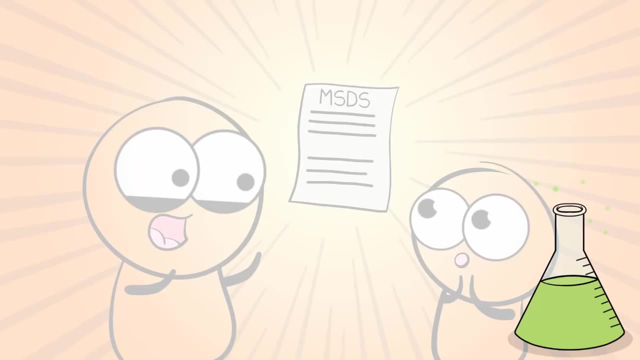 extinguisher and or a fire blanket in the room. finally, the MSDS. it stands for material safety data sheet. it's available for pretty much every substance you use in your lab. you should refer to it because it will give you all kinds of safety information on a substance, including how to safely handle.